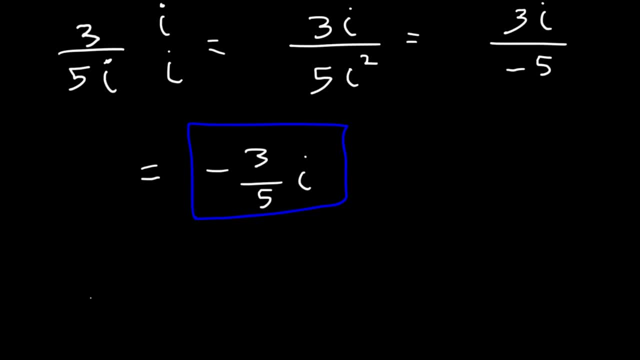 So now it's in standard form. Standard form is a plus bi. In this problem, a is 0. So it's a minus 3 over 5 times i, or 0 minus 3 over 5 times i. So how can you convert this expression to standard form? Let's say, if we have 4 plus 2i divided by 3i, 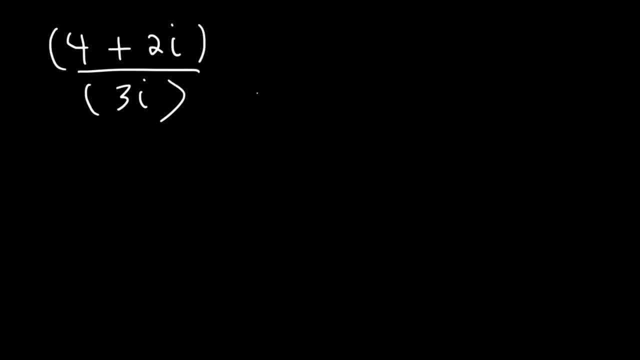 So first we need to get rid of the imaginary number in the bottom. So let's multiply the top and the bottom by i. So on top it's going to be 4i plus 2i squared. On the bottom we're going to have 3i squared. 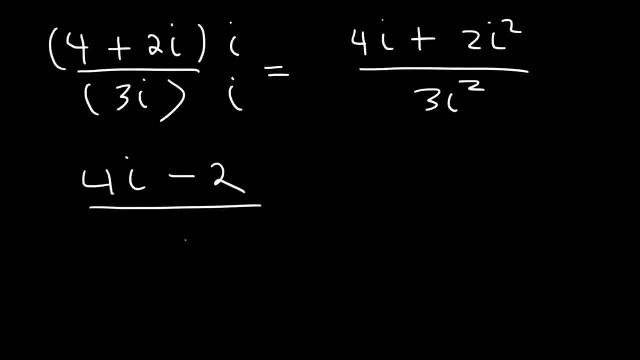 2i squared is equal to negative 2. 3i squared is negative 3.. So we're going to divide both numbers by negative 3.. So negative 2 divided by negative 3 plus 4i divided by negative 3.. 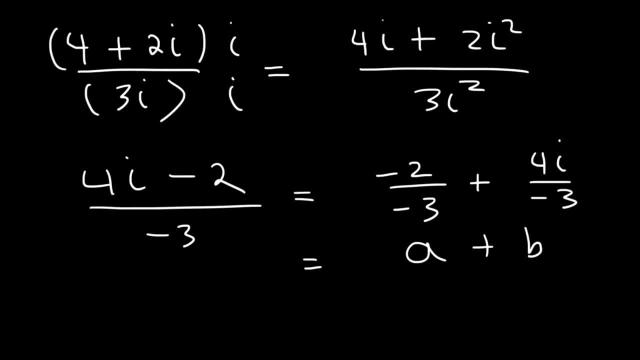 So in standard form, that is, in a plus bi form, a is positive, 2 over 3.. The two negative signs will cancel. b is negative, 4 over 3, and then times i. So that's the answer. Go ahead and rationalize the denominator, Get rid of the radical and the imaginary number. 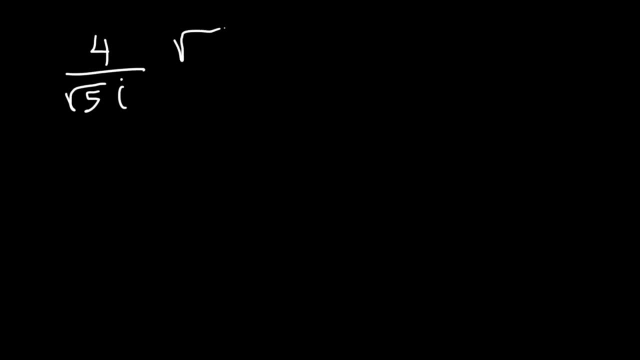 So to simplify this particular problem, we need to multiply the top and the bottom by root 5.. So on top it's going to be 4 root 5 times i. On the bottom, root 5 times root 5 is 5.. i times i is i squared. 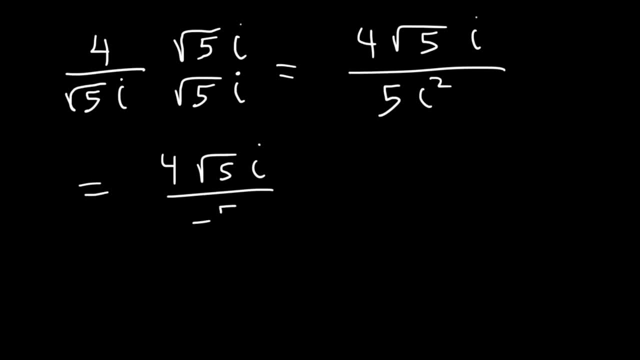 So 5i squared is equal to negative 5.. So in a plus bi format it's 0 minus 4 over 5 root 5 times i. Now, what about this one? Go ahead and simplify this problem: 8 divided by 3 plus 2i. 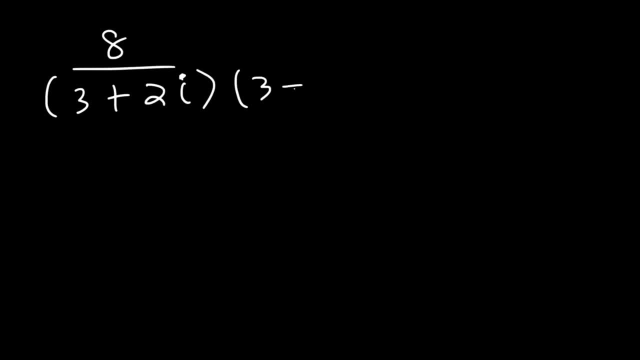 So if you have two terms on the bottom, multiply the top and the bottom by the conjugate of the denominator. The conjugate of 3 plus 2i is 3 minus 2i. You simply have to change the sign. So, on top, let's distribute the 8.. 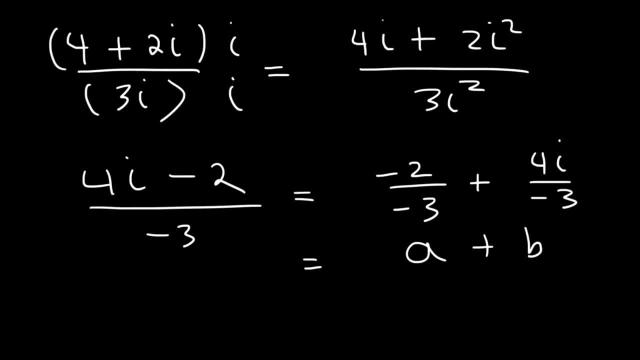 So in standard form, that is, in a plus bi form, a is positive, 2 over 3.. The two negative signs will cancel. b is negative, 4 over 3, and then times i. So that's the answer. Go ahead and rationalize the denominator, Get rid of the radical and the imaginary number. 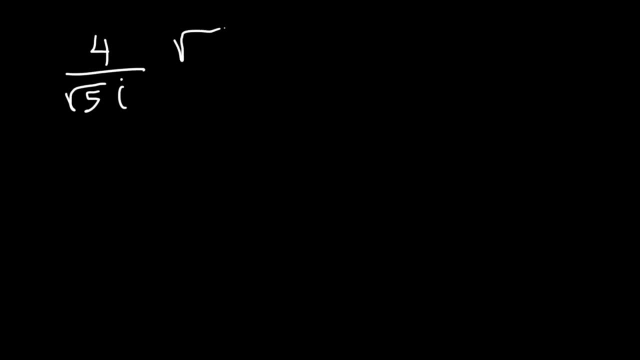 So to simplify this particular problem, we need to multiply the top and the bottom by root 5.. So on top it's going to be 4 root 5 times i. On the bottom, root 5 times root 5 is 5.. i times i is i squared. 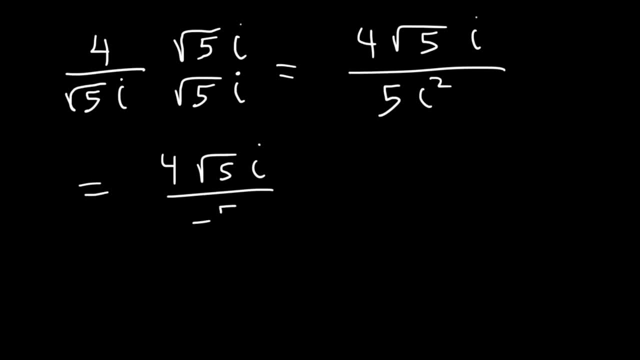 So 5i squared is equal to negative 5.. So in a plus bi format it's 0 minus 4 over 5 root 5 times i. Now, what about this one? Go ahead and simplify this problem: 8 divided by 3 plus 2i. 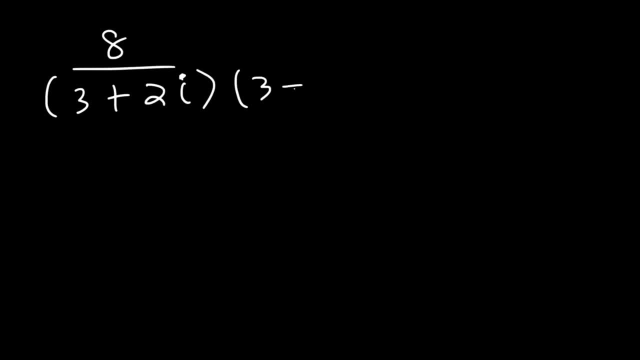 So if you have two terms on the bottom, multiply the top and the bottom by the conjugate of the denominator. The conjugate of 3 plus 2i is 3 minus 2i. You simply have to change the sign. So, on top, let's distribute the 8.. 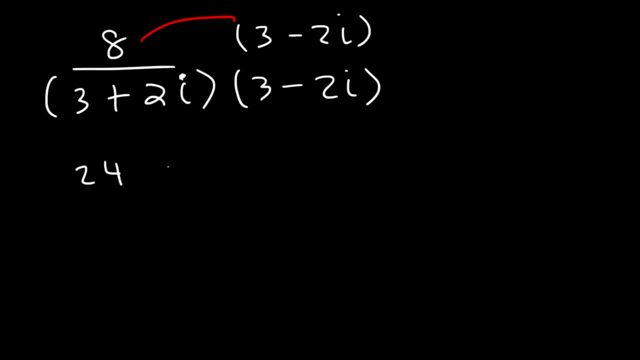 8 times 3 is 24.. 8 times negative 2i is negative 69.. On the bottom, let's FOIL. We know the two middle terms will cancel. 3 times 3 is 9.. 3 times negative 2i is negative 6i. 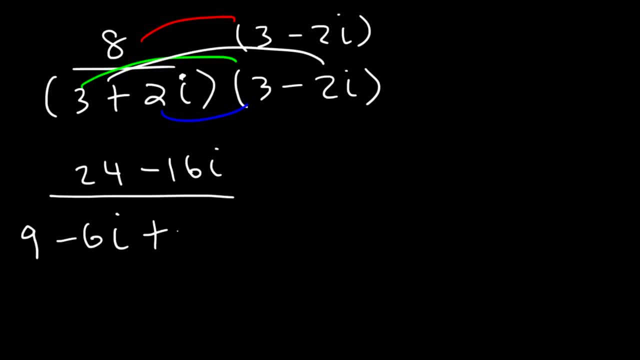 And then 2i times 3,, that's positive 6i. And then 2i times negative, 2i is negative 4i. squared Now, the two middle terms adds up to 0. And so it's 24 minus 16i. 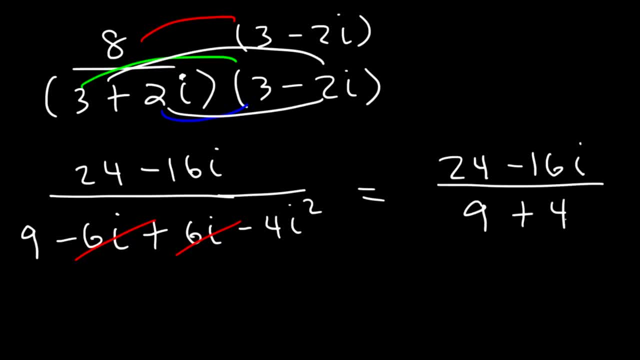 Negative 4i squared is plus 4i, Because i squared is negative 1. And 9 plus 4 is 13. So we can write it as 24 over 13 minus 16 over 13i. Now it's in standard form. 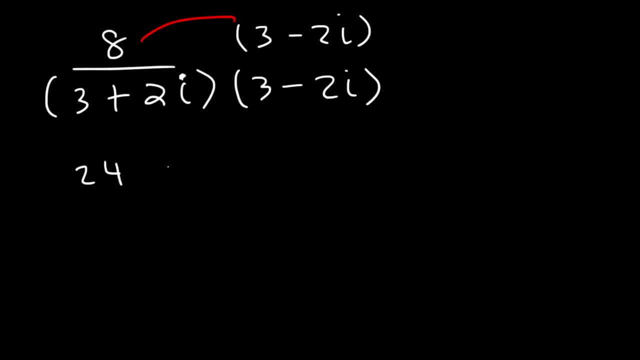 8 times 3 is 24.. 8 times negative 2i is negative 69.. On the bottom, let's FOIL. We know the two middle terms will cancel. 3 times 3 is 9.. 3 times negative 2i is negative 6i. 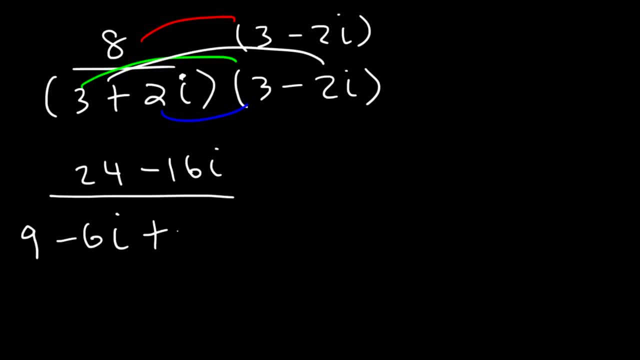 And then 2i times 3,, that's positive 6i. And then 2i times negative, 2i is negative 4i. squared Now, the two middle terms adds up to 0. And so it's 24 minus 16i. 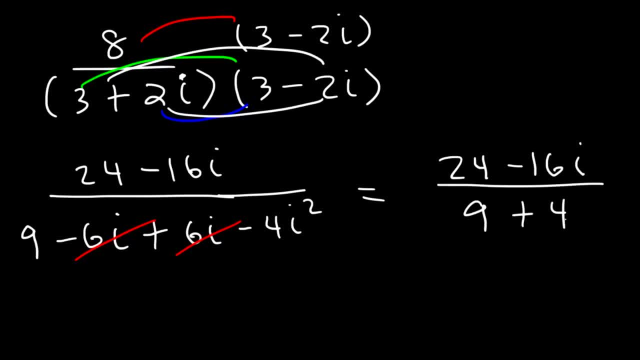 Negative 4i squared is plus 5i 4 because I squares negative 1, and 9 plus 4 is 13, so we can write it as 24 over 13 minus 16 over 13. I now it's in standard form. let's try one more example. 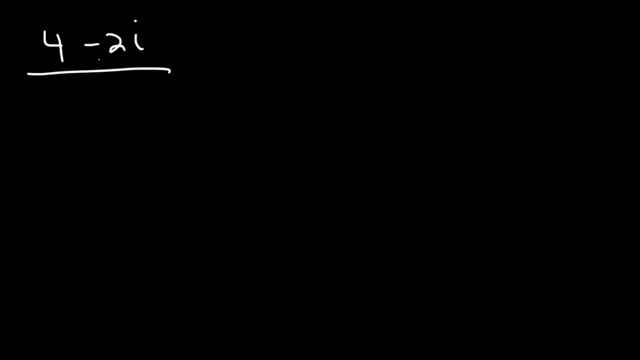 4 minus 2, I divided by 3 plus 5. I simplify the expression. so we're gonna have to multiply the top and the bottom by the conjugate of the denominator. so on top we need to foil 4 times 3. that's going to be positive 12, and then 4 times. 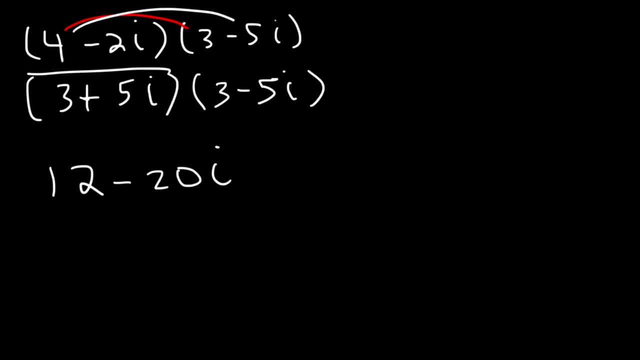 negative 5 I, that's negative 20 I. and then negative 2 I times 3, that's negative 6 I. and then we have negative 2 I times negative 5 I. that's going to be positive 10. I. squared on the bottom. the two middle terms will cancel, so what's gonna be left over is 3. 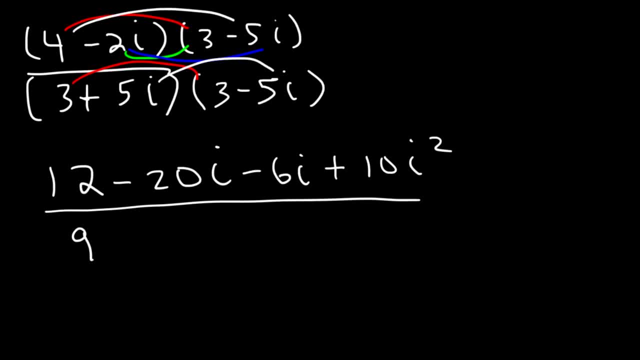 times 3, which is 9, and also 5 I times negative 5 I, which is negative 25 I squared. so in the numerator let's combine the like terms. so it's 12 minus 26 I and 10 I squared is negative. 10 negative 25 I squared, that's gonna be. 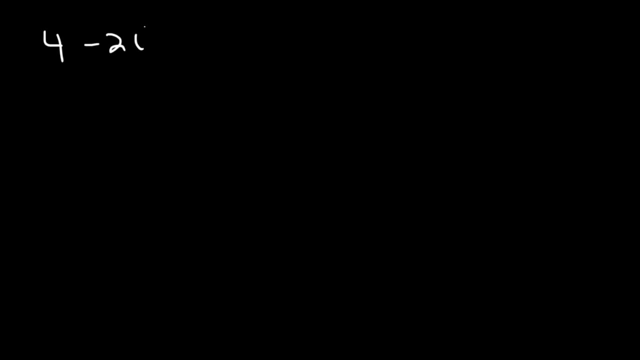 Let's try one more example: 4 minus 2i divided by 3 plus 5i Simplify the expression. So we're going to have to multiply the top and the bottom By the conjugate of the denominator. So on top we need to FOIL. 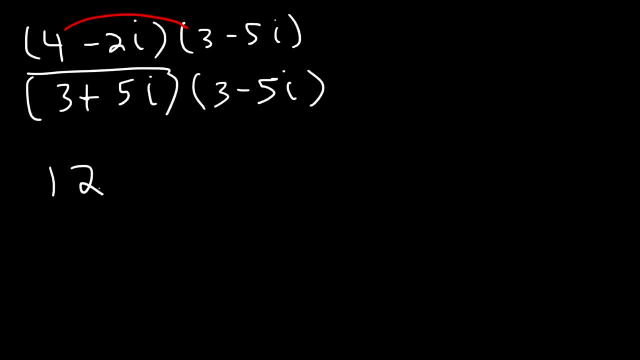 4 times 3,, that's going to be positive 12.. And then 4 times negative 5i, that's negative 20i. And then negative 2i times 3,, that's negative 6i. And then we have negative 2i times negative 5i. 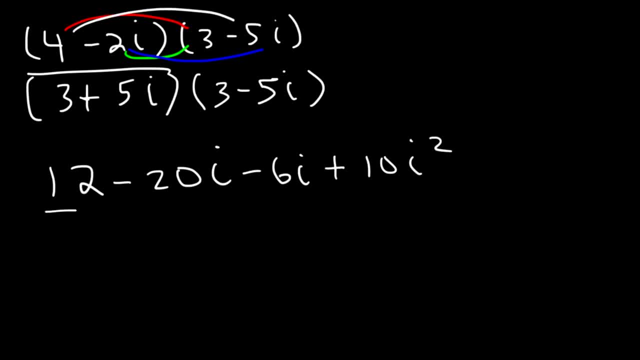 That's going to be positive: 10i squared. On the bottom, the two middle terms will cancel. So what's going to be left over is 3 times 3,, which is 9.. And also 5i times negative, 5i, which is negative. 25i squared. 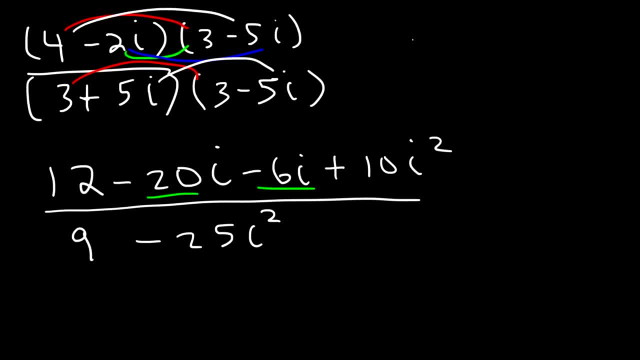 So in the numerator let's combine the like terms. So it's 12 minus 26i And 10i squared is negative 10.. Negative 25i squared, that's going to be positive 25.. 12 minus 10 is 2.. 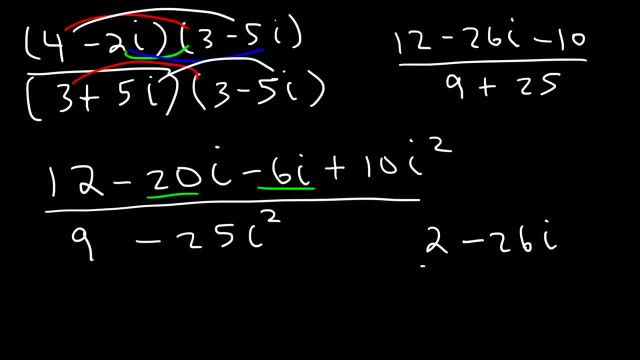 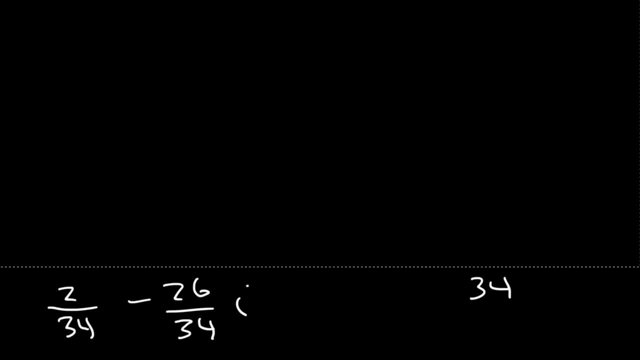 9 plus 25 is 34.. So we can separate into two fractions, 2 over 34 and negative, 26 over 34 times i. Now let's simplify the fractions 2 over 34,. if you divide both numbers by 2, it reduces to 1 over 17.. 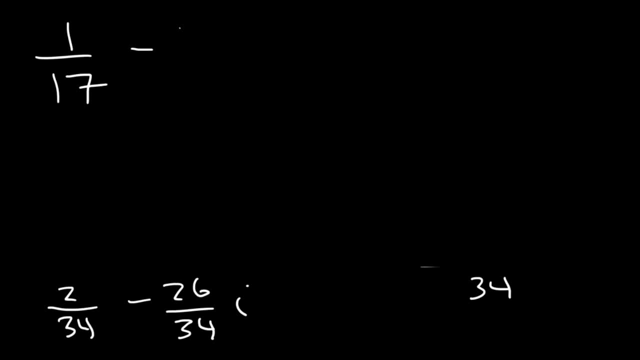